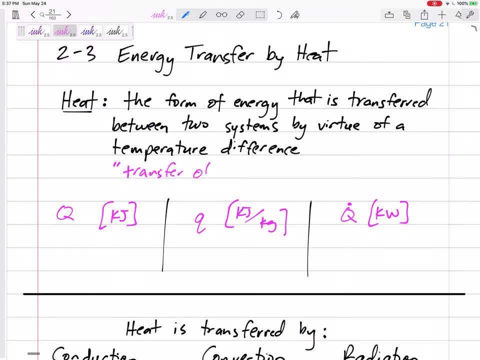 energy. Heat is a transfer of thermal energy, So it's almost heat energy or thermal energy. It's really a transfer of thermal energy because of a temperature difference. If there is no temperature difference between an object and its surroundings, then it doesn't give off any heat. 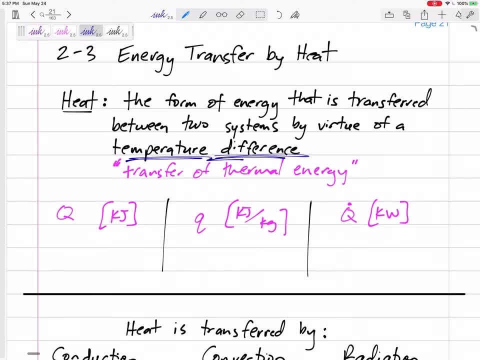 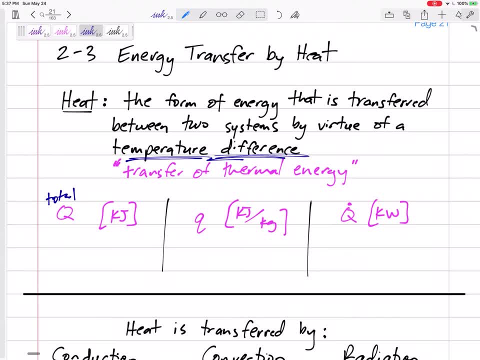 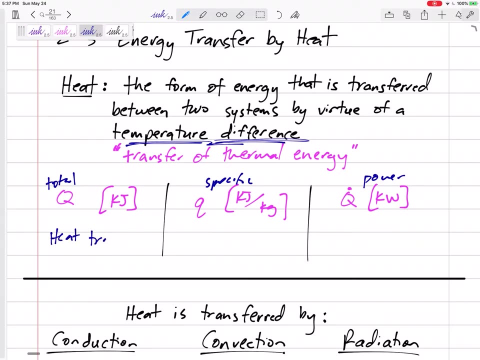 it could be total heat transfer. It could be specific, It could be the power. We could look at the units or the variables. So if we are thinking about the heat transfer, or the heat transfer per unit mass or the heat transfer per unit time, then we'll denote those by 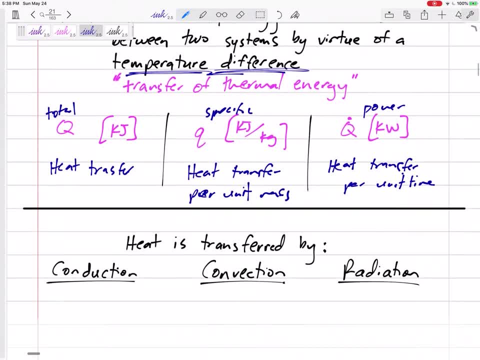 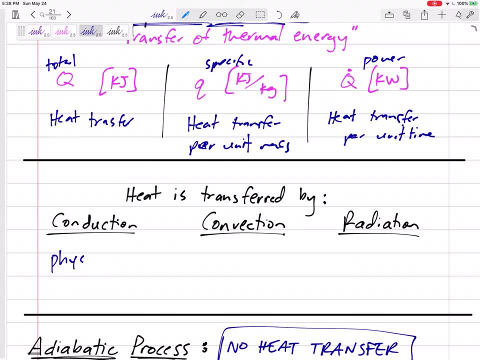 q's and the units will be pretty important. All right, heat can be transferred by conduction. convection, radiation. You all have heard this before. right, Conduction is like physical touch, two things touching each other. Convection is fluid motion and radiation is electromagnetic waves. 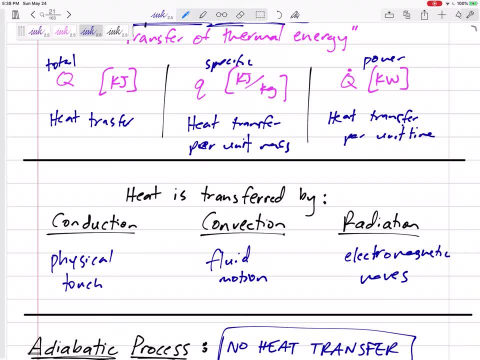 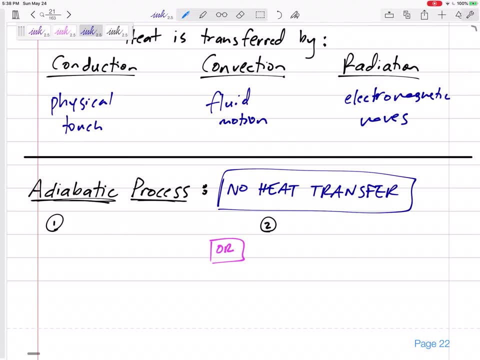 All right, so three different ways heat can be transferred. Now our definitions: if something is adiabatic, then there is no heat. There is no heat transfer. right, Q is zero. So if it says it's adiabatic, then Q is zero, that there is no heat transfer. 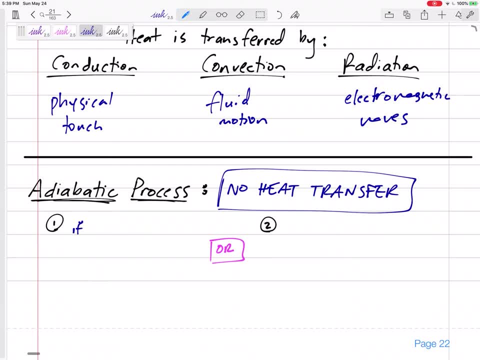 Or it probably may not say adiabatic, It might say the system is well insulated. So if the system is well insulated, then what it's really telling you is there's no heat transfer. Or if the system, If the system and the surroundings are at the same temperature, then there's no Q. 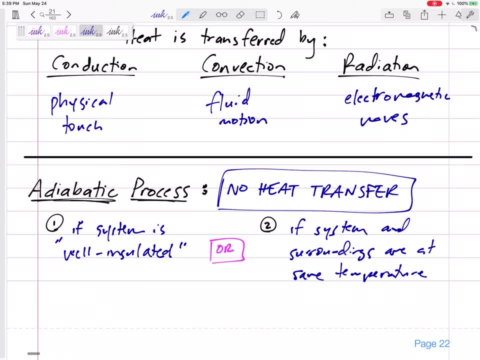 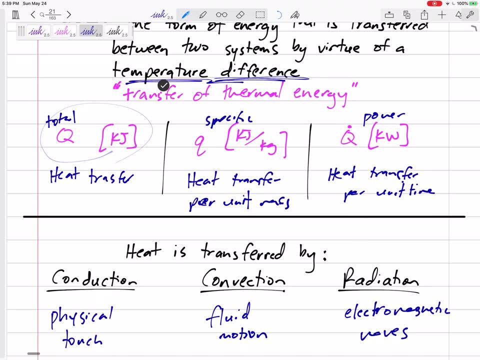 There's no heat transfer, Don't have to calculate, Don't have to worry about that. Okay, So right now we don't have an equation for Q. We will just need to kind of be told the heat transfer. maybe we can calculate the Q. 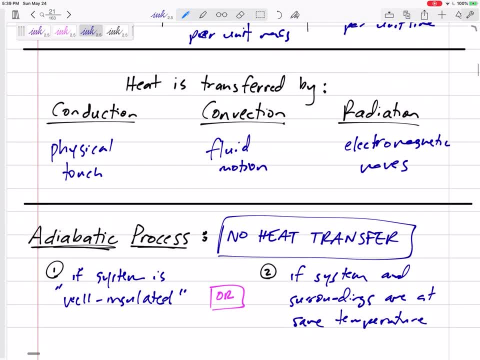 Depending on whether it's asking for total, specific or power. 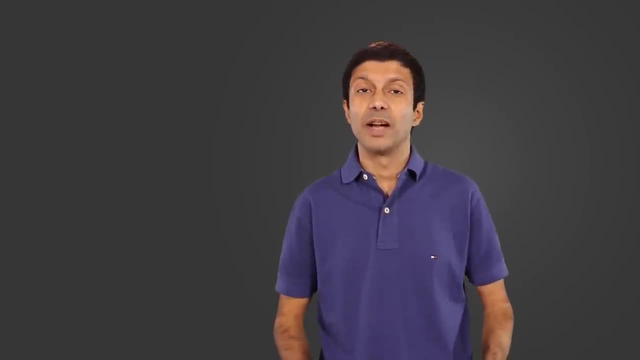 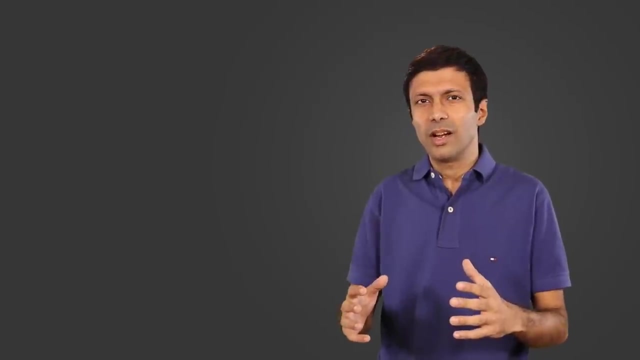 A few days back, I went swimming with my daughter. My daughter is 4 years old and she is learning to swim, So you can imagine how the swimming session went right. Most of the time I am holding her up in the pool and she is enjoying herself. So while holding her in water, I realized 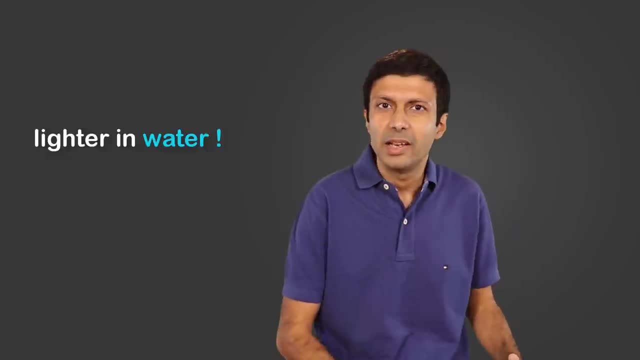 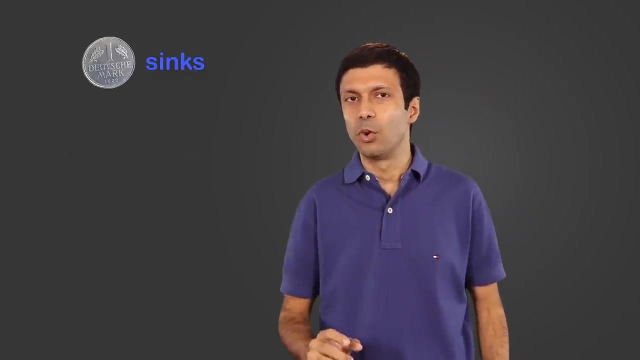 that she feels much lighter in water than when I lift her up at home. So how can you explain that? That's right, it's Archimedes' principle, And this same principle explains why a small steel coin sinks in water, but a massive steel ship can float. But before. 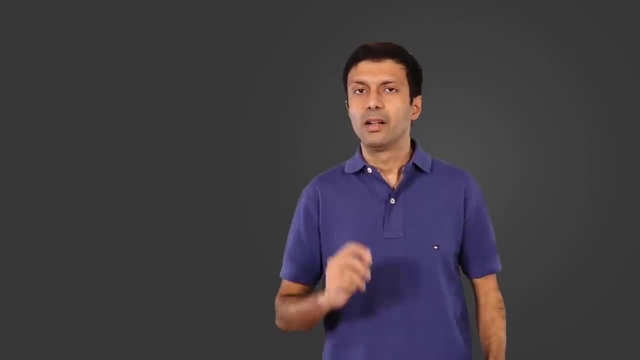 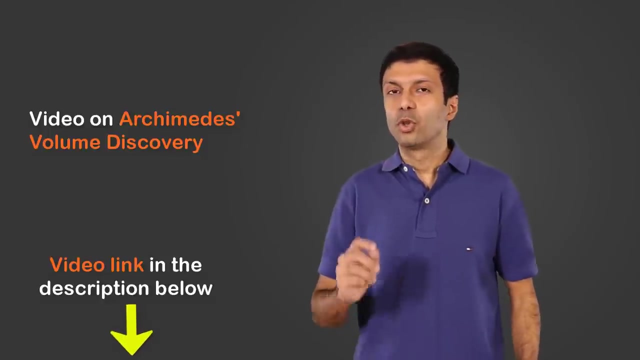 we do Archimedes' principle. you need to understand Archimedes' volume discovery. I have a video on Archimedes' volume discovery so if you've not watched that already, do check it out. I'll be posting the link in the description. 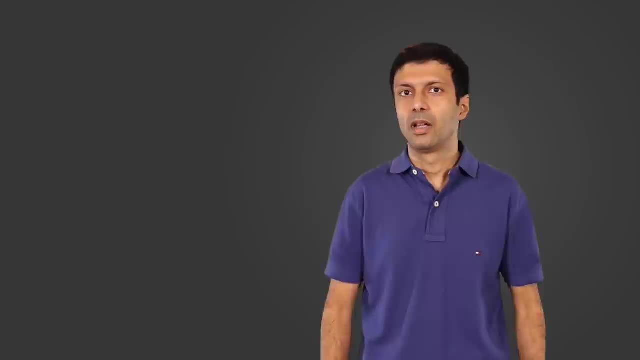 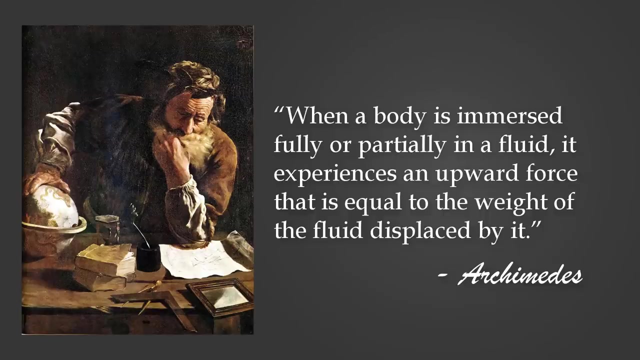 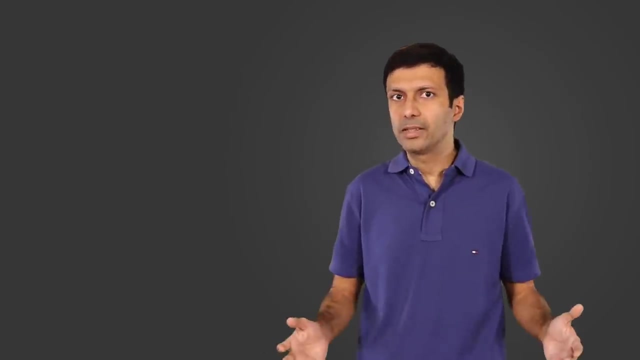 Now, if you look up Archimedes' principle in the textbooks, Archimedes said: When a body is immersed fully or partially in a fluid, it experiences an upward force that is equal to the weight of the fluid displaced by it. The first time you read this it sounds like a cryptic message from Archimedes. 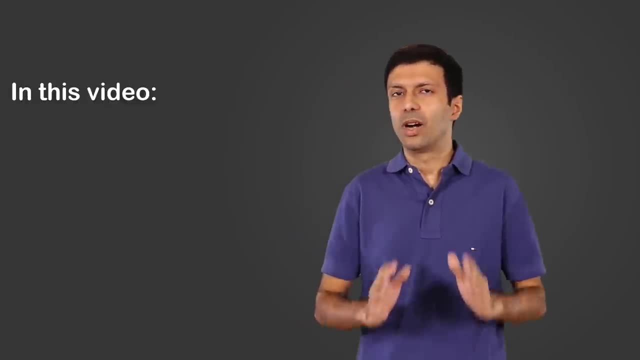 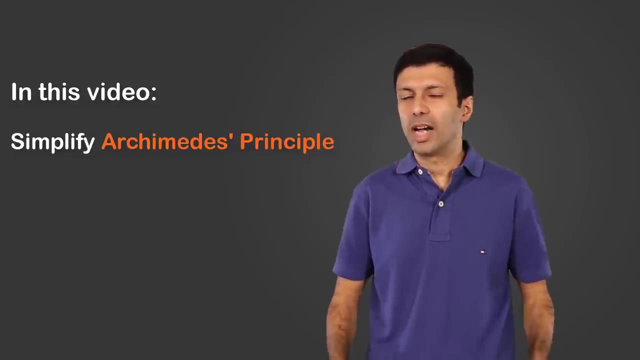 But don't worry, Archimedes' principle is true. Archimedes' principle is true In this video. I'm going to break it down and really simplify it for you. Also, towards the end of the video, I'll be sharing a great mnemonic to help remember this principle. 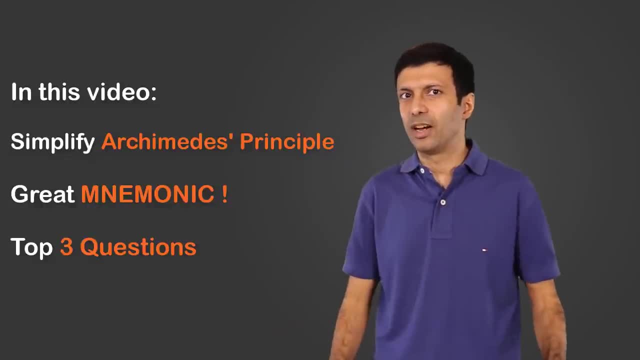 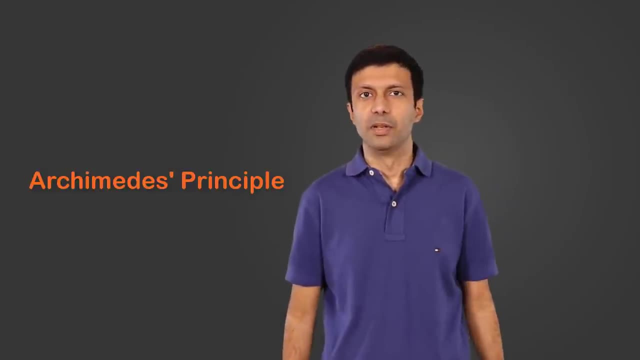 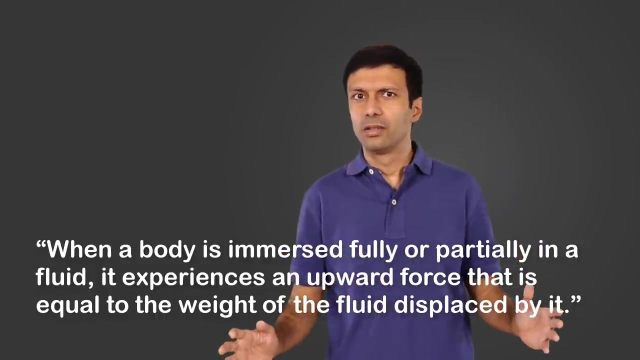 So do stay tuned, And then we'll finish off with our top 3 questions on this topic. Let's start with Archimedes' principle. So here's the statement: 1., 2., 3., 4., 5..